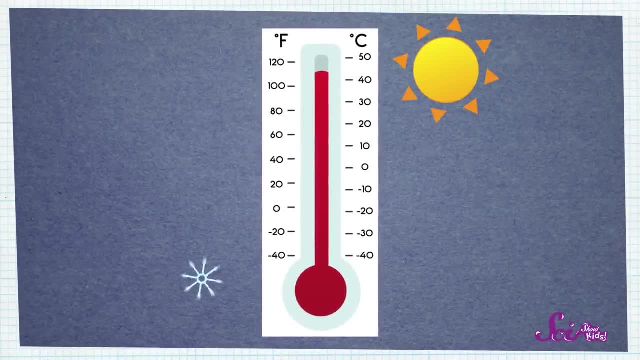 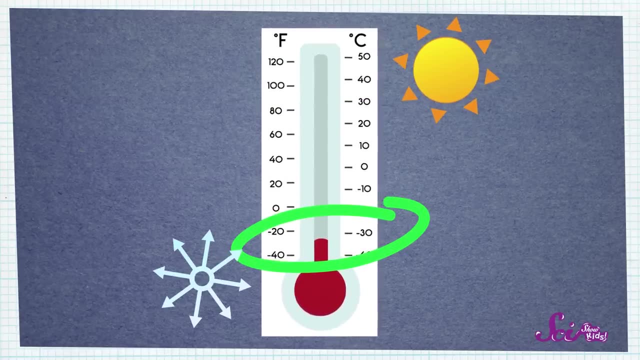 It tells you what the temperature is outside, how hot or how cold it is. The higher the liquid is inside of the thermometer, the hotter it is outside, And the lower the liquid is, the colder it is outside. If you want to keep a weather journal, like I do, then you might want to see if your family 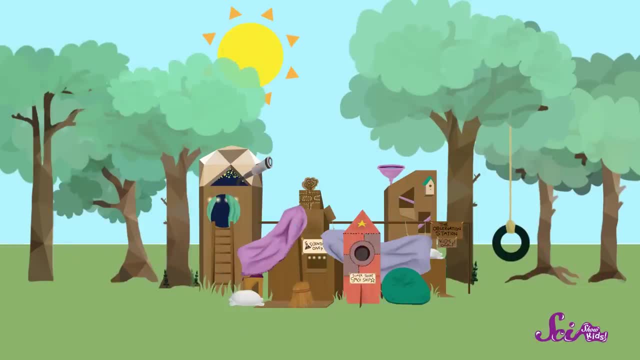 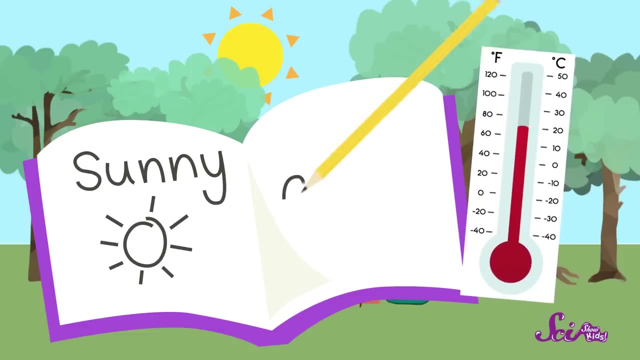 can get an outdoor thermometer to help you record the temperature. Then every day you can look outside and write down what you see Or draw a picture. Next, look at the temperature on your thermometer And write down what you see. Write down how hot or cold it is. 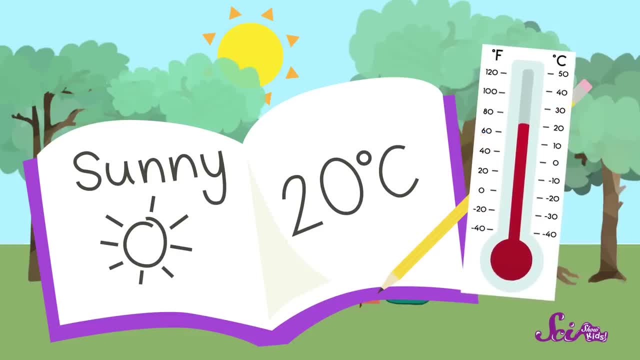 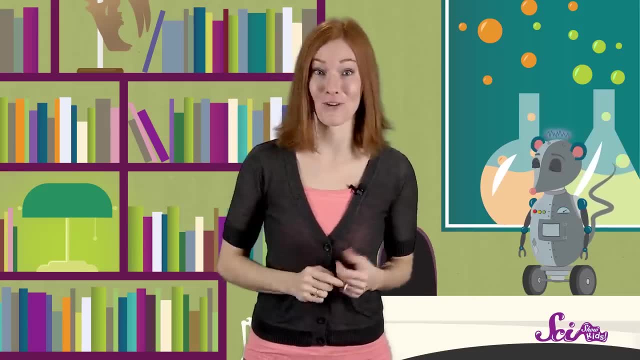 Just look for the line on the thermometer that's closest to the top of the liquid. That's your temperature. I like to write in my weather journal at the same time every day, right after breakfast. You can pick a time that works best for you and observe the weather at the same time every. 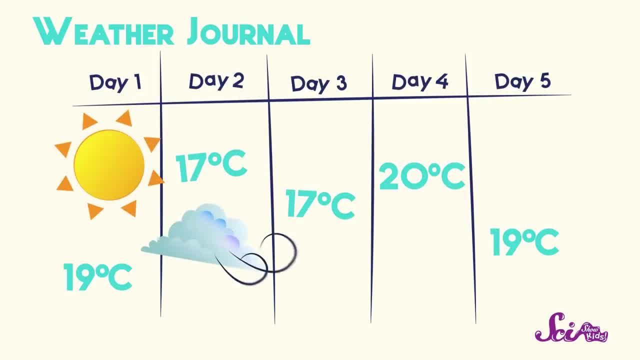 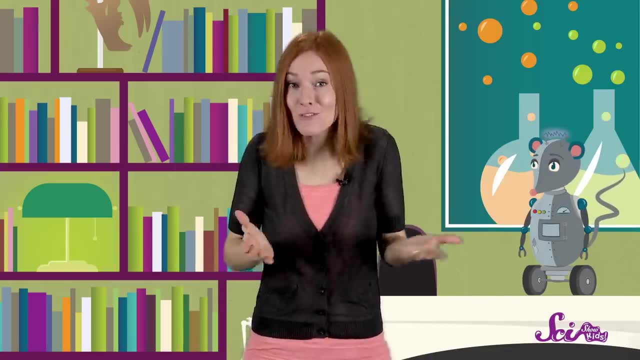 day for five days. After five days, look back through your weather journal. What was the weather like this week? Did you see any patterns? Can you guess what the weather might be like on the sixth day based on what you've seen already? Share your journal with your friends and, if you want, you can keep observing the weather for more than five days. If you watch the weather for, say, a whole month, you'll be able to watch the weather change. In fact, you'll probably see at least a few of the different types of weather that. 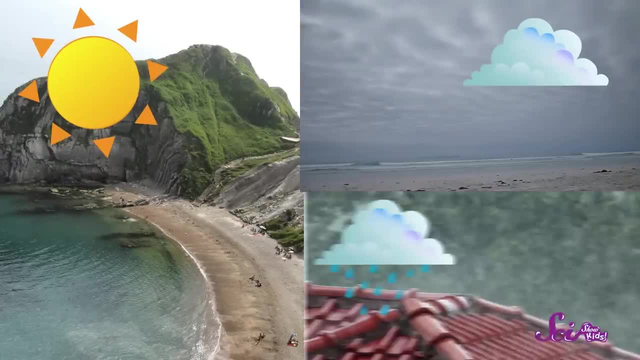 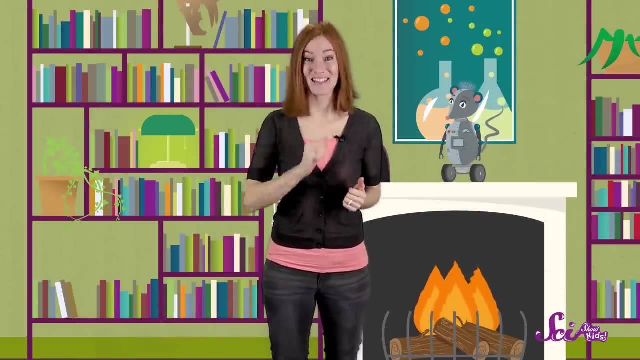 we talked about earlier- a mix of sunny, cloudy and rainy days- And if you keep your weather journal for a whole year, you'll be able to see the weather where you live at its hottest and its coldest, And you'll have a list, either in your words or your pictures, of everything that happened. 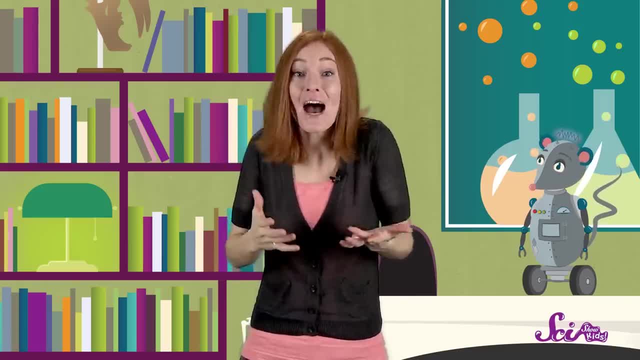 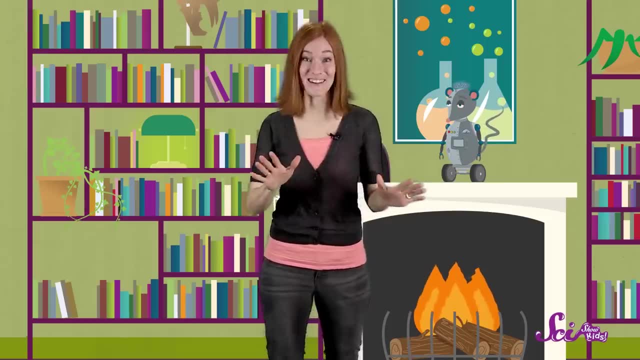 that year. Then you'll know when the first snow of the winter was, Then the highest and lowest temperatures of the year, and if it rained more some times of the year than others. So grab your notebook and get outside. it's time to watch the weather. 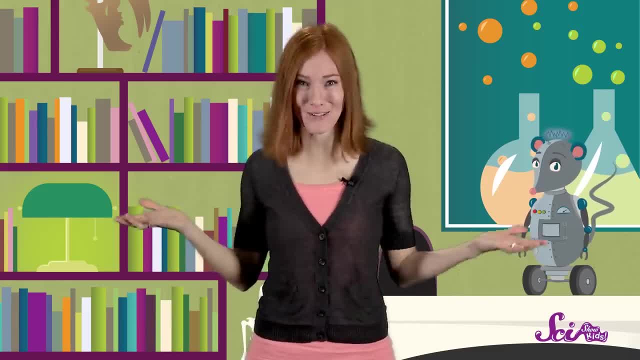 Thanks for joining us on SciShow Kids And remember, if you have a question for any of us here at the Fort, let us know by leaving a comment or emailing us at kids at thescishowcom, and we'll see you next time. Subtitles by the Amaraorg community. 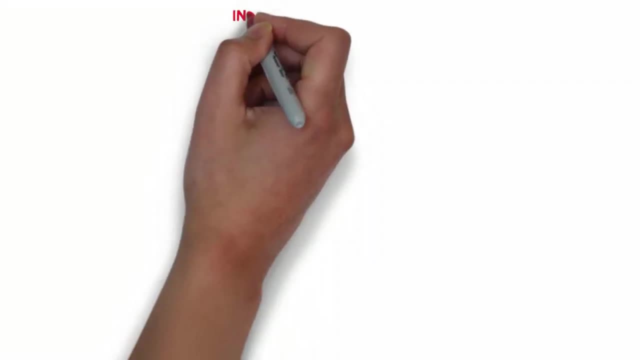 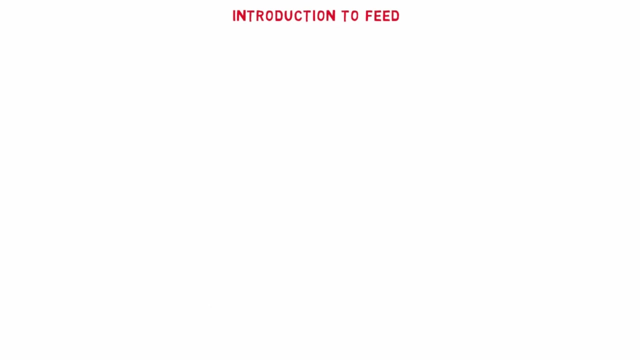 Hello friends, welcome to our channel, Piping Mantra. In this video we are going to discuss briefly about FEED in perspective of piping. So let's discuss about what is FEED. FEED stands for Front End Engineering Design. The FEED is basic engineering, which comes after.